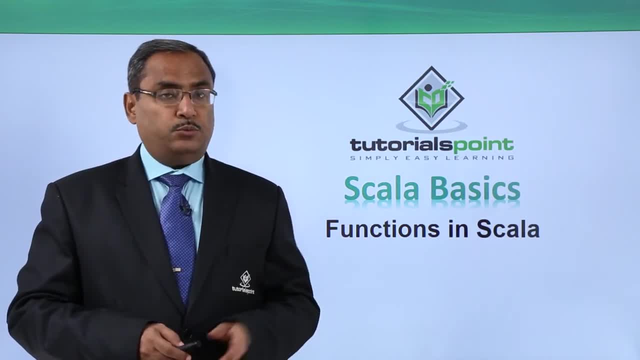 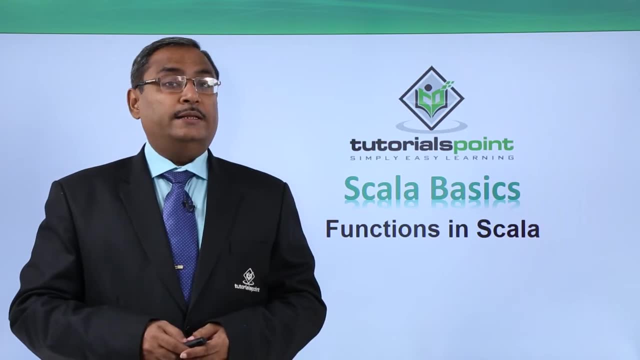 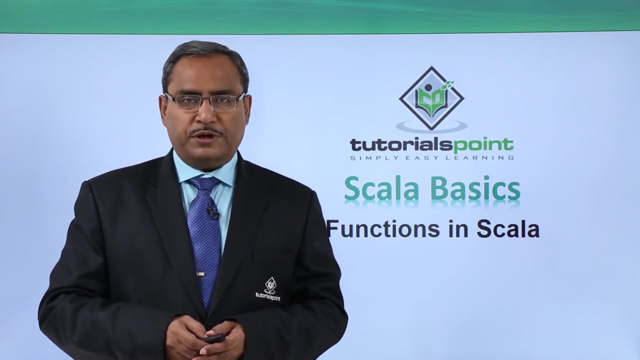 Functions in Scala. We are starting with a new chapter with this video, that is, our Scala functions. So in case of Scala, we can write functions, and these functions can be of different types. So let me discuss what are the different features we are going to cover in this very chapter. 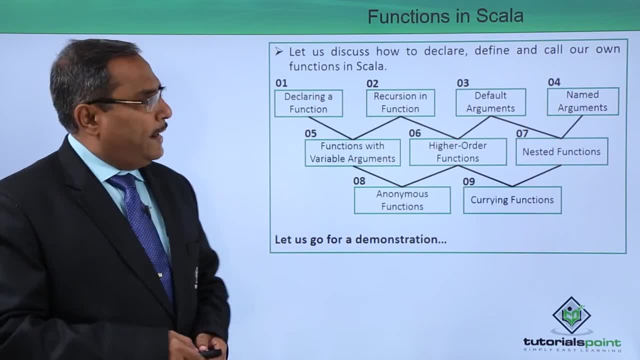 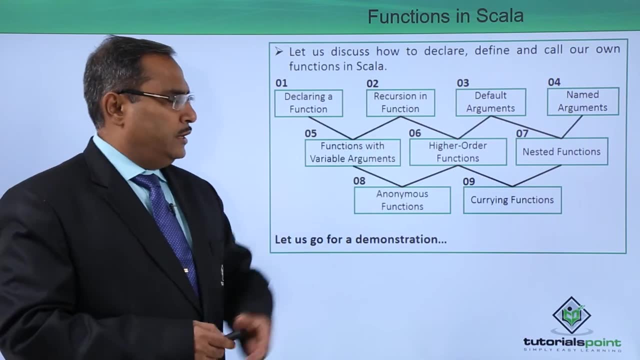 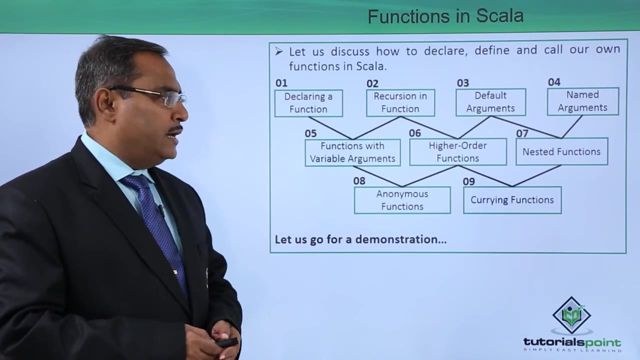 So let us discuss how to declare, define and call our own functions in our Scala programming. So declaring a function, recursion in function function with the default arguments and then named arguments, We are having functions with variable arguments, high order functions. we 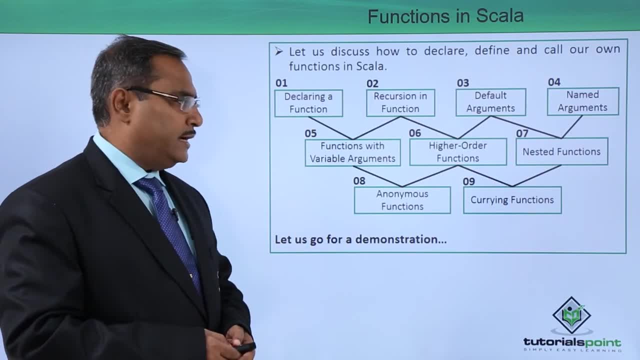 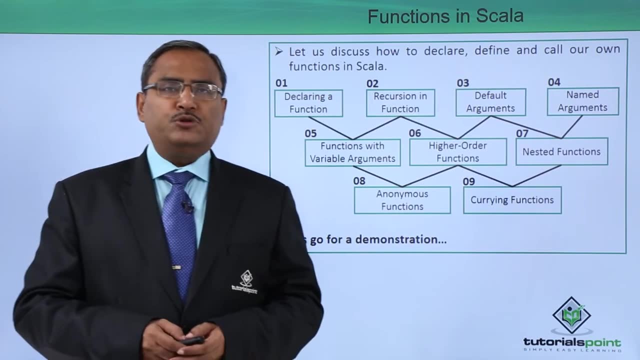 will be discussing nested functions, anonymous functions and cutting functions, So so many different features will be covered in this respective chapter. Right now we are going for one demonstration to show you how to declare one function, how to write one function and how. 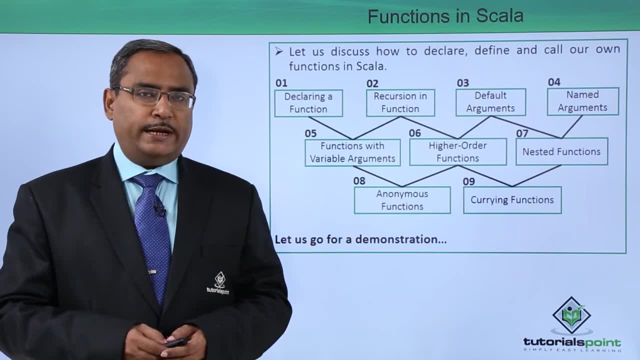 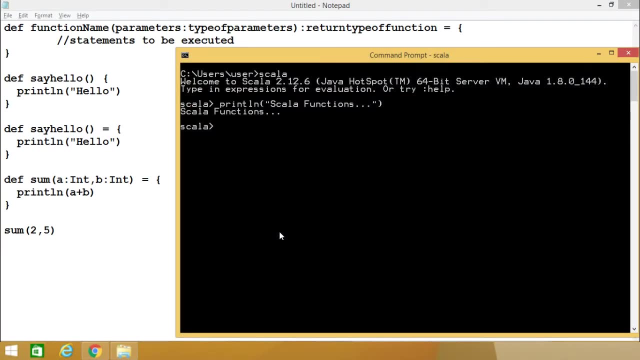 to call it- and during execution. So let us start with the demonstration- how the outputs are getting produced. So here is the demonstration. In this session we are going to discuss introduction to Scala functions. and when we want to execute a group of statements to perform a certain task for, say, hundred number of times, we usually don't type the 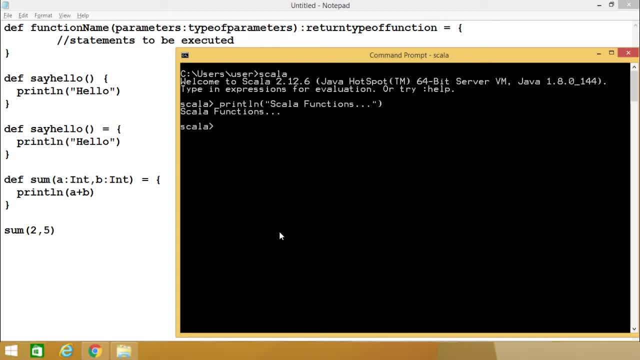 code for 100 times. obviously we group them into a function and we shall put a call to that function inside a loop and we shall make the loop rotated or make the loop executed for, say, 100 number of times. dividing our code into functions also makes our code more modular, so you are bringing modularity. 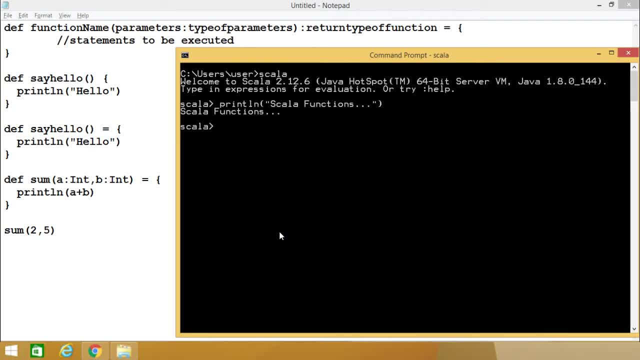 in our code, which will help us for the easier debugging and for the modification of the code, and we can do this division according to the tasks we carry out in our code. so Scala is rich in built-in functions and it it is also lets us create our own user different functions. 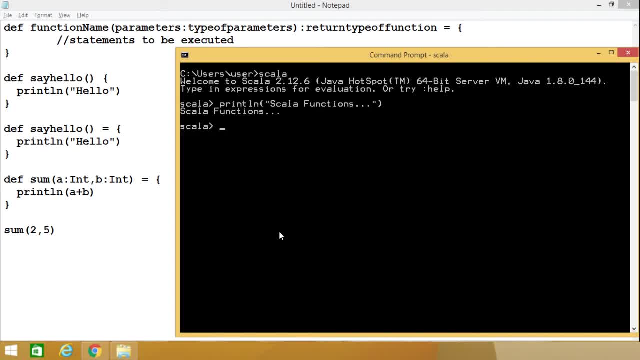 so here Scala functions are known as the first class values. so Scala also has methods, but these differ only slightly from the respective Scala functions. a method belongs to a class or a one object, and these particular methods will be denoting the behavior of the class or the. 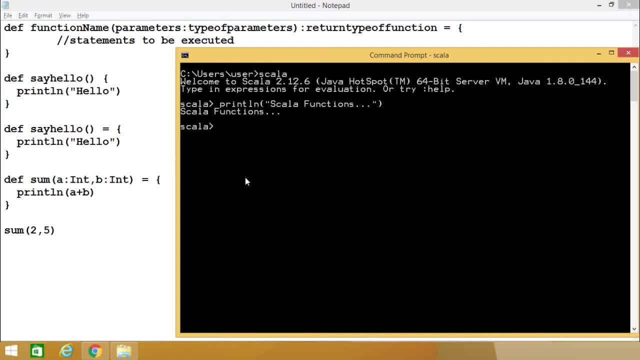 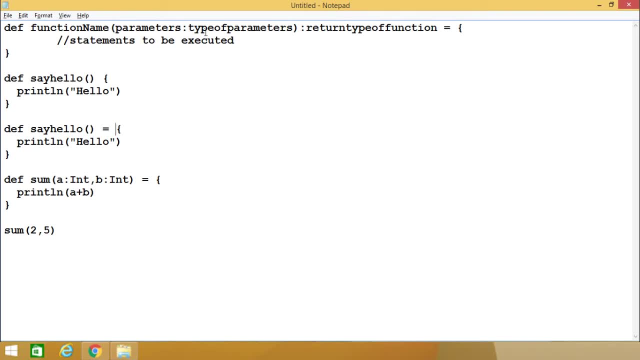 respective object here. so what is the basic syntax of writing Scala functions, so def: function name. this is a list of parameters, input parameters and the respective type of the parameters, and then colon, then return type of the function. so respective type, return type of the function should be mentioned after colon. then 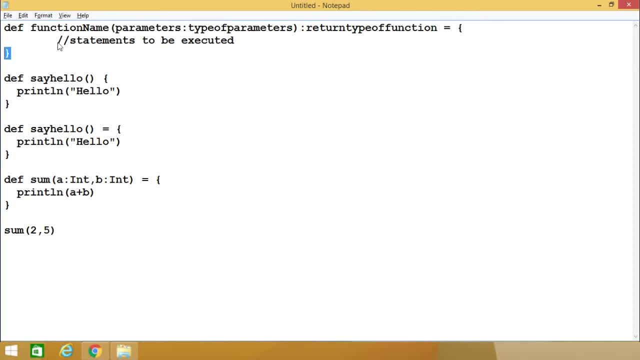 equal to then, within the calibres, will be writing the respective statements to be executed. so now let us show you that how these codes are getting executed. so here we are having a def, there is a definition. then we are having this: say hello, hey is a particular function. so say hello is a function. 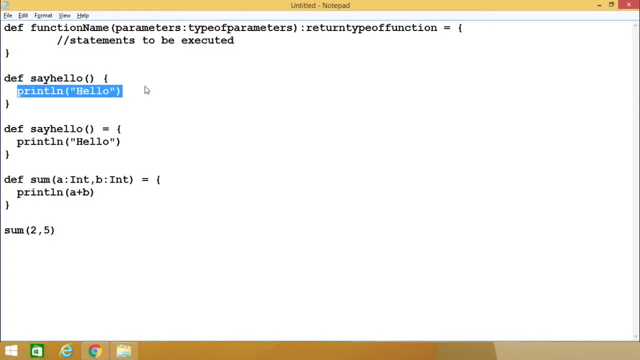 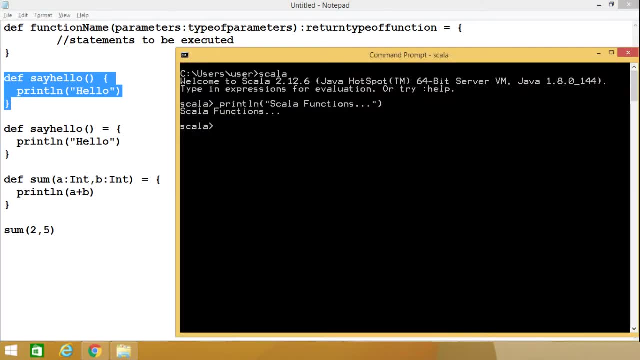 which is having a single code here. so single statement is there. so println hello. and within the curly braces the function body has got written. so I'm just making a copy and here I'm going for this interactive shell, I'm pasting it here. so here you see, the function has got defined and that is our say hello. function has got defined. 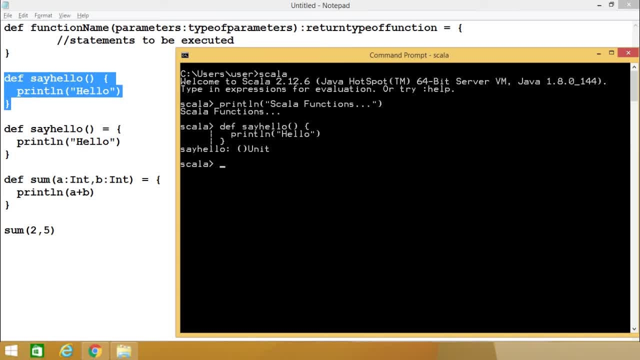 and it returns unit. that means it returns void, as we didn't mention any any kind of return and data type. so that's why it is taking that it returns nothing, or it returns unit or void. so now let me call this function. so I'm calling this function here, so hello is getting printed as: 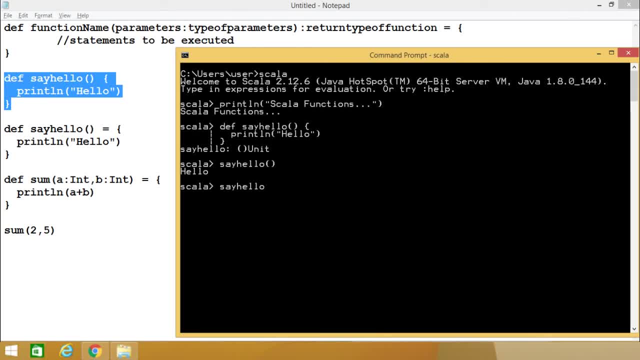 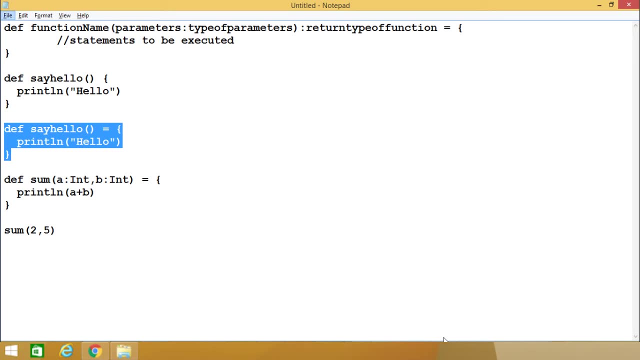 this function is not having any input parameter, so also without this- first brackets, opening and closing also- you can call it and it will work accordingly. now let us suppose we are putting one equal to symbol, so I'm just copying it and showing you that the same code will get executed. 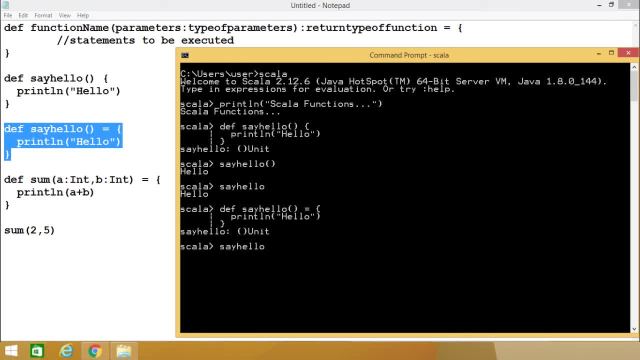 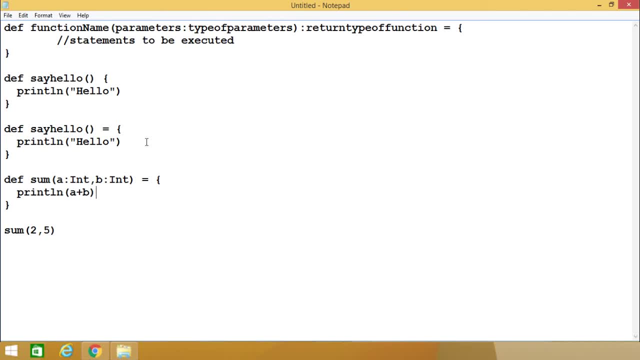 the same code has got executed. so here I'm just going for this say hello. I'm going for this say hello in this way. so codes are working fine. now what will happen if we pass some input arguments? so here you see, here we are passing some input arguments here, so I'm just copying the code. 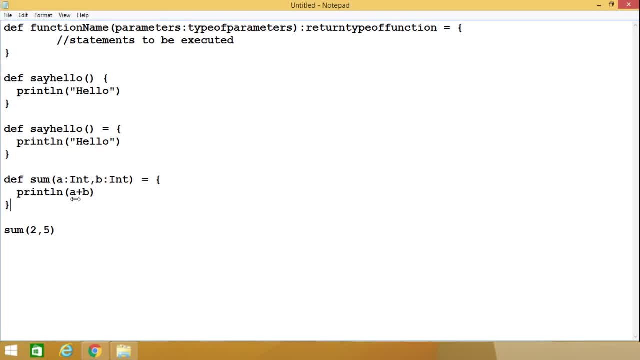 so here you see, here we are having. this name of the function is sum, and it is taking two input arguments, a and b, of type integer. it returns nothing, so that's why we haven't mentioned anything here- and then print l and a plus b will be the respective output. so now, if I execute this, 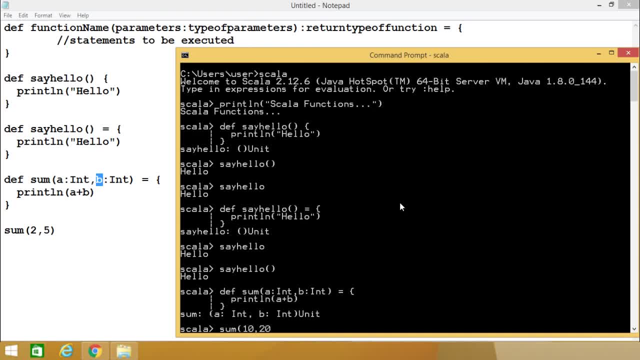 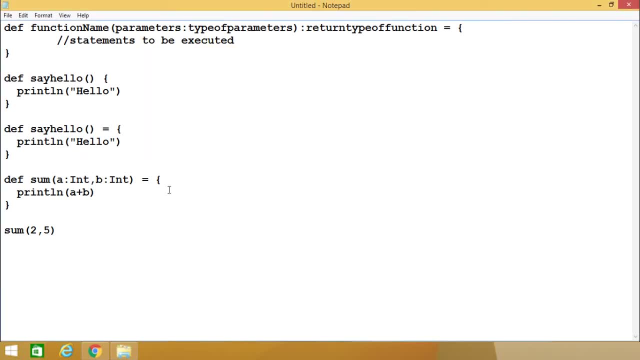 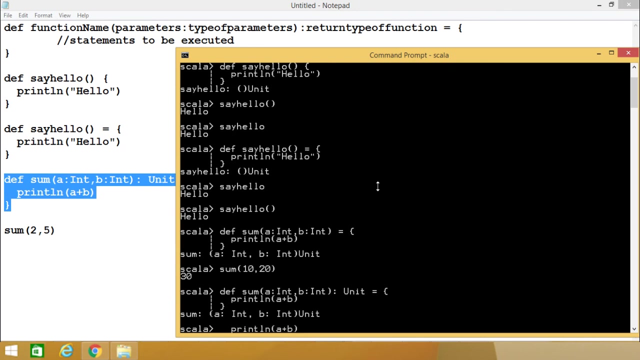 one. so I'm sure I shall call this one with the value set 10 and 20. if I call this one, then I'm getting 30 here. so here also, we can write here unit. we can write here unit as it returns nothing. so here you see the. you can call it now. so now it is getting executed as well. so here in this video,